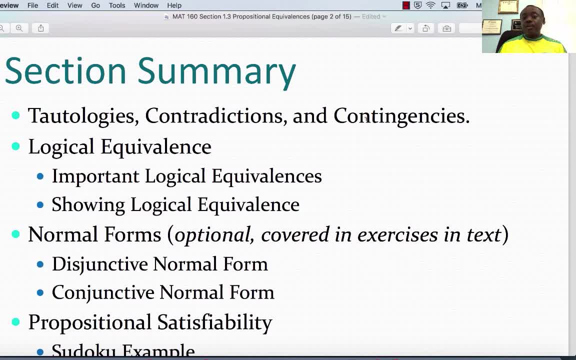 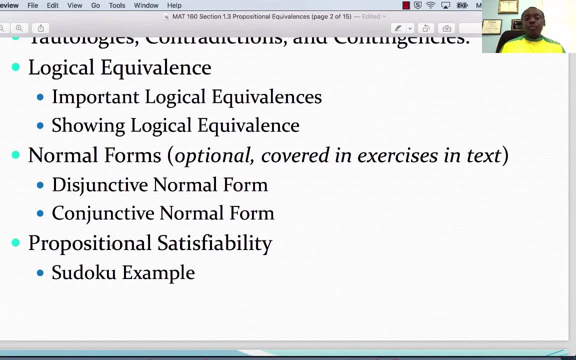 look at tautologies, contradictions and contingencies. Then we would move down to logical equivalence and look at some important logical equivalences and how to show logical equivalences, And then we would skip right down to propositional satisfiability. Now let's go. 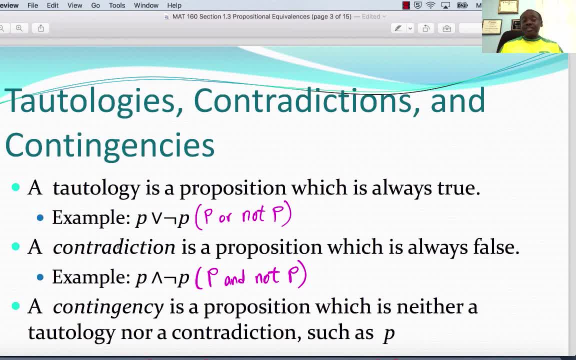 ahead and start. Definition, Tautologies, contradictions and contingencies. A tautology is a proposition which is always true, For example, P or not? P is always true. He ate a slice of pizza did not eat a slice of pizza. that is always true. a contradiction, on the other hand, is a proposition. 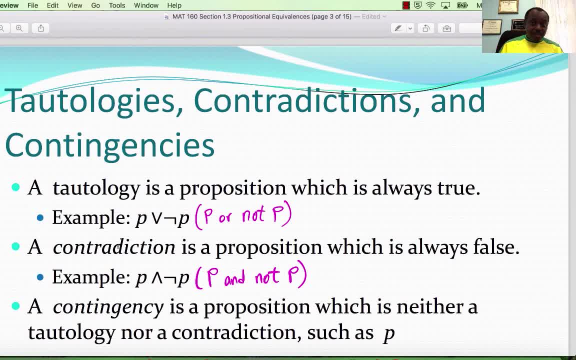 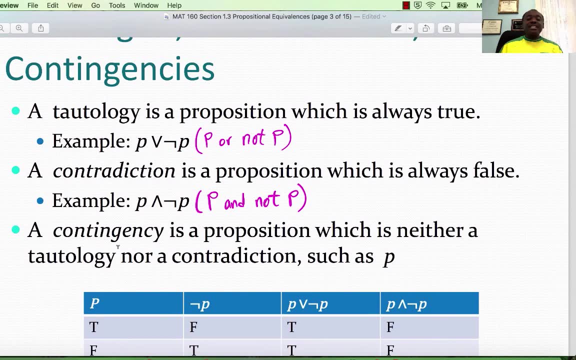 which is always false. for example, p and not p. he had a slice of pizza and he did not eat a slice of pizza. it's a problem contradiction, it's always false. and thirdly, we have a contingency. a contingency is a proposition which is neither a tautology nor a contradiction, it's just a. 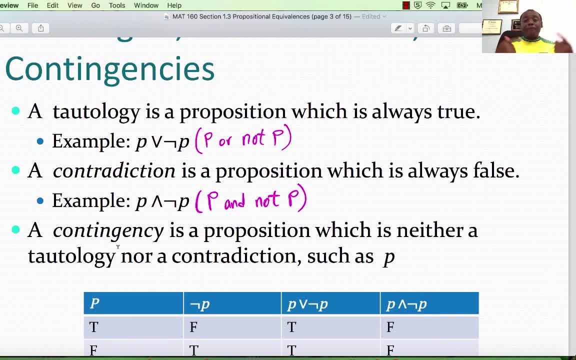 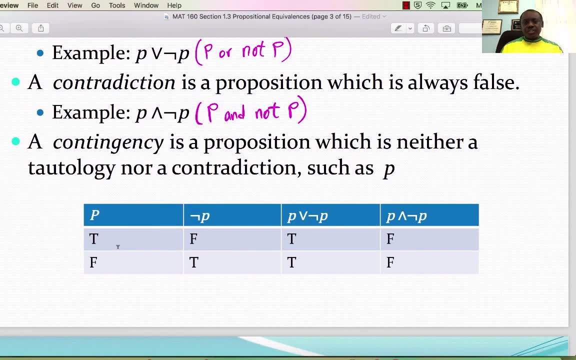 proposition. it could be true or false, depending on more information. so, for example, p, he played soccer this morning. we need more information before we can conclude whether it's t or f. now let's look at the truth. tables for contradictions and tautologies. so we have p. 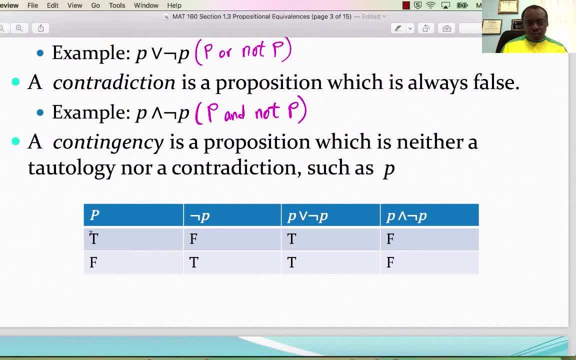 and we have not p again. just one proposition. so two truth values on the column, and p or not p. we end up with t, t or true. so that means a tautology: p and not p. we have f, f and that means a contradiction. okay now. 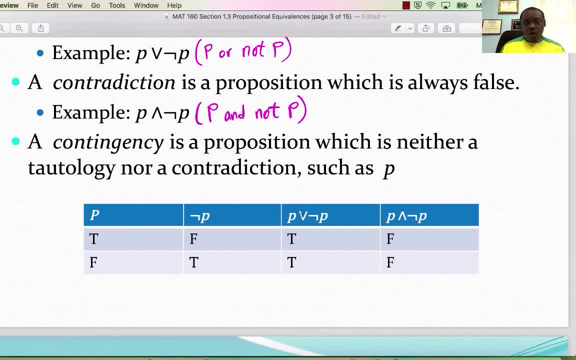 recall two tables. we've done this before. all is true. if any one of them is true, it's only false. if both are false, and we don't have that situation, so it's all true. and on the other hand, it's only true if both are true, otherwise false and we do not have that situation, so it's all false. 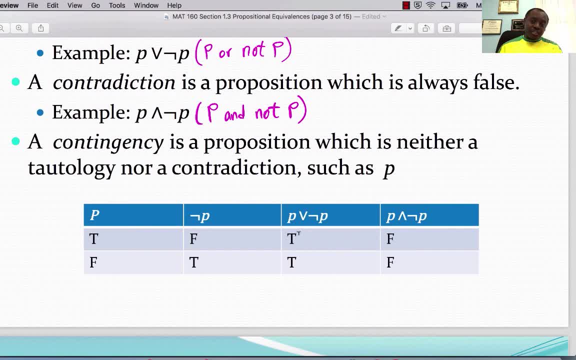 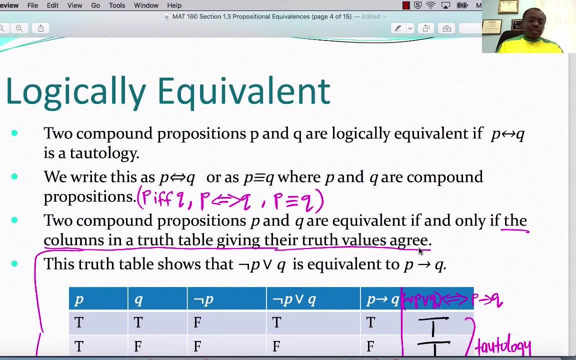 so here we have a tautology and here we have a contradiction. all true and all false. now let's move on to the next objective in section 1.3: logical equivalence. how do we prove or how do we show that two propositions are logically equivalent? well, two compound propositions p. 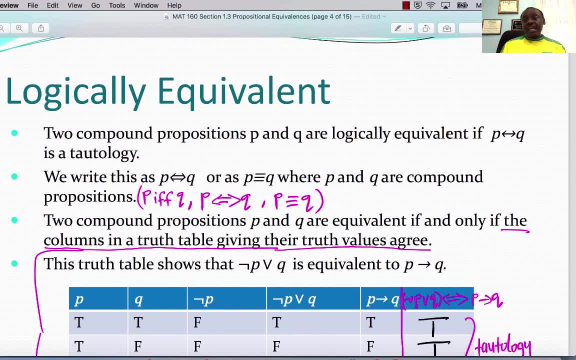 and q are logically equivalent. if the biconditional p, if and only if q is a tautology, we can also represent that with p, if and only if q or p is equivalent to q, where p and q are compound propositions. additionally, we can also say that two compound 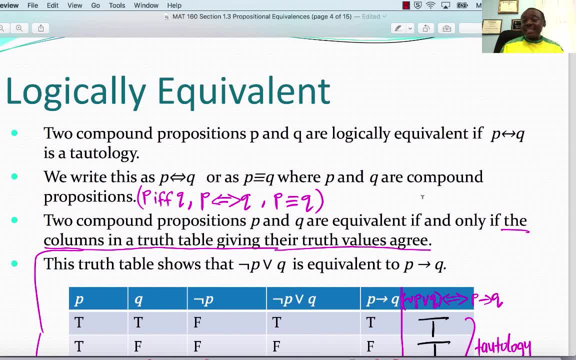 propositions p and q are equivalent if, and only if, the columns in a truth table, given their truth values, agree. so two compound propositions are equivalent if, and only if their respective columns agree. so there are two ways to prove that two compound propositions are logically equivalent. number one: we can show that p if, and only if, q is a tautology. number two: we can 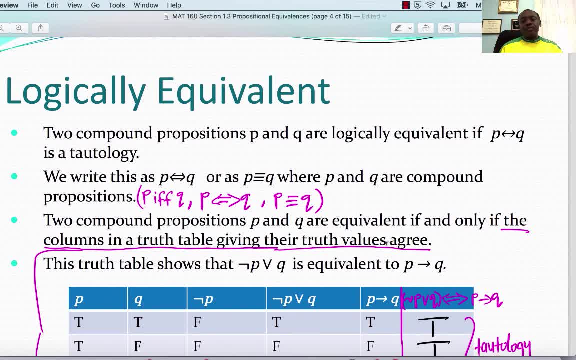 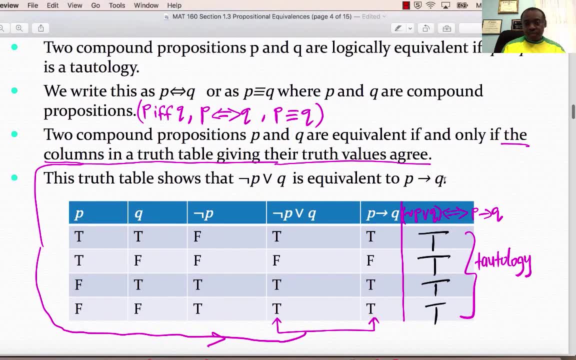 show that the two columns that give the truth values of these propositions agree. let's go ahead and verify that for these two propositions right here. one is not p or q. p implies q. we claim that p implies q is logically equivalent to not p or q, by the way. we establish. 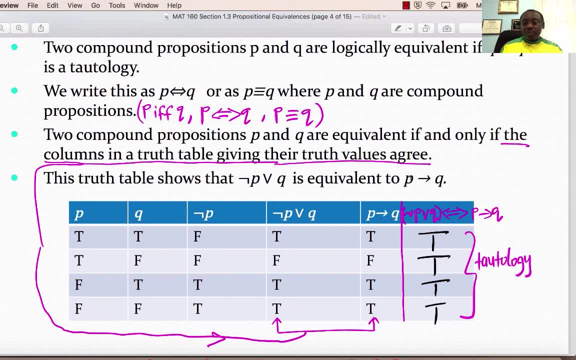 logical equivalence, we can always replace p implies q with not p or q, and vice versa. so that's why we are interested in logical equivalence, because if i have p implies q, i can simply write it as not p or q, and it would still be the exact same thing. so 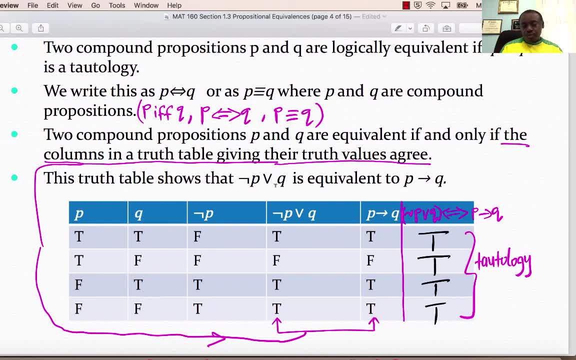 let's verify that. we have two propositions. so we're looking at two to the two, which is four truth values. here we are: that's p, that's q. we have not p. and then we go with this first guy right here, the first compound proposition: not p or q, not p or q gives us this column and we move on to p. implies 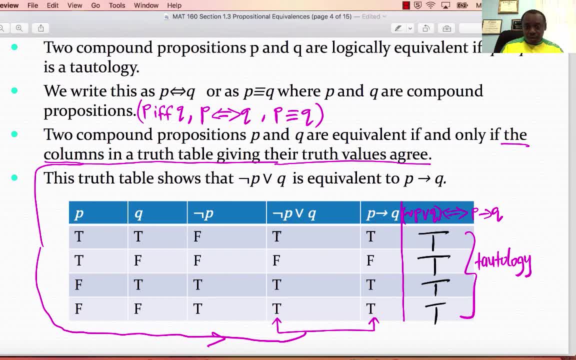 q. it gives us this column right here and we observe that this column not p or q. the other column, p, implies q. the truth value is not p or q and we observe that this column not p or q. the other values agree. so we can stop right here and conclude that these two compound propositions. 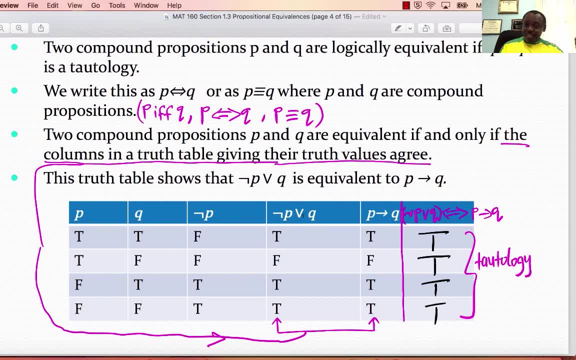 are equivalent, but we said something about tautology, so we could also do not p or q, if and only if, p implies q, and recall that if and only if is true, if and only if, both truth values are the same. so t and t is t, f and f is t, and if, and only if, is true, then both truth values are the. 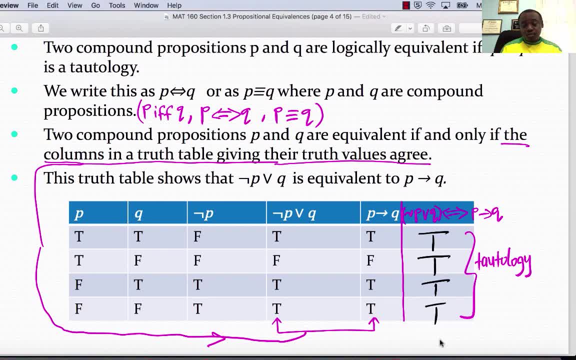 same. so t and t is t, t and t is t- all true. that is a tautology. so if you did not want to conclude using the fact that these truth values agree, you could just go down here and look at the last column and say that, because we have a tautology, the compound proposition, not p or q, is logically. 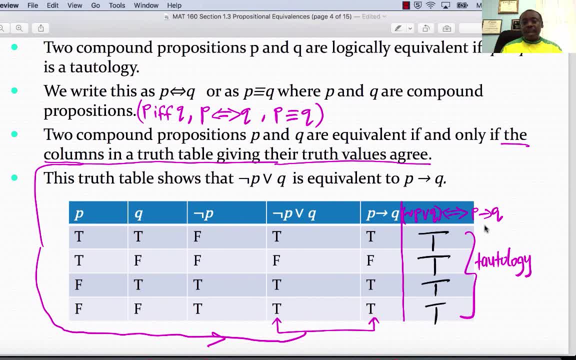 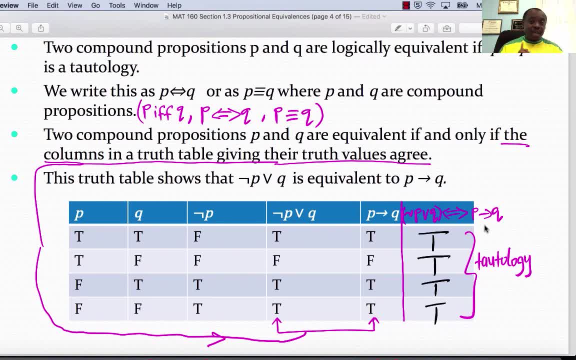 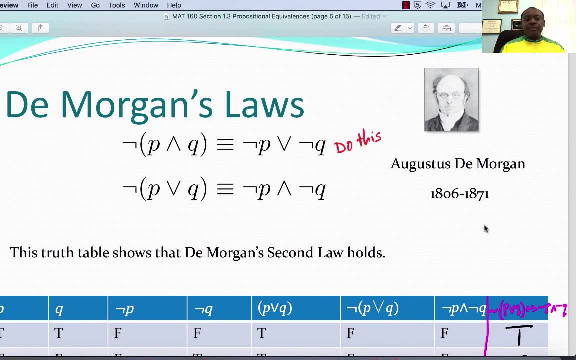 compound propositions are logically equivalent without using a truth table. augustus de morgan, 1806 to 1871, gave us what is known as de morgan's laws is very popular. you see that in set theory, in logic, almost everywhere we have de morgan's laws. it claims number one that not p and q is equivalent to not p or not q. 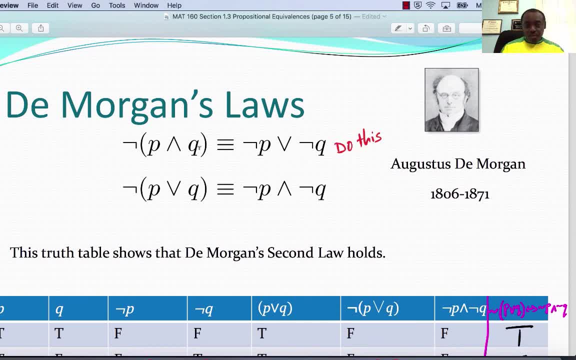 the and changes to all, and both propositions are negated. the second one: the all changes to and, and both propositions are negated. so prove that this compound proposition is logically equivalent to this and this compound proposition is also logically equivalent to this. we're going to do one of them and you would do the other one on your own. let's look at: 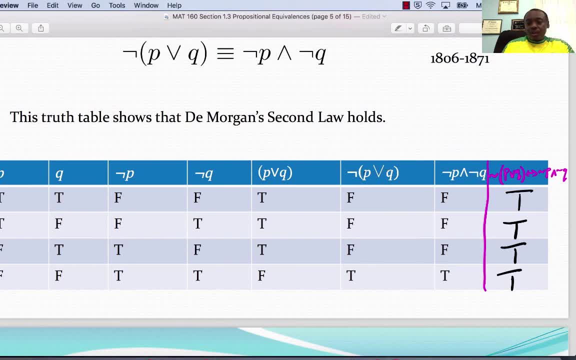 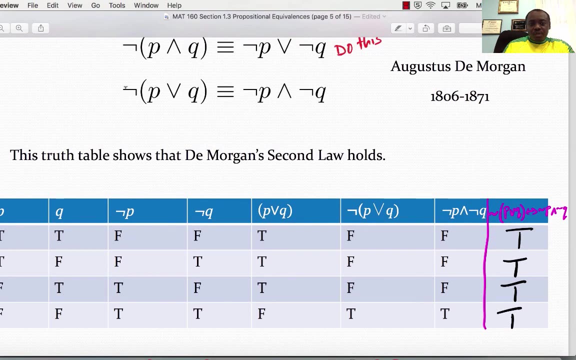 not p or q. de morgan claims that not p or q is logically equivalent to not p and not q. well, if you do your truth table, we have p, we have q, we have not p, we have not q. and because we are going to deal with not of all of this, so we start off with p or q and then negate the second one and then 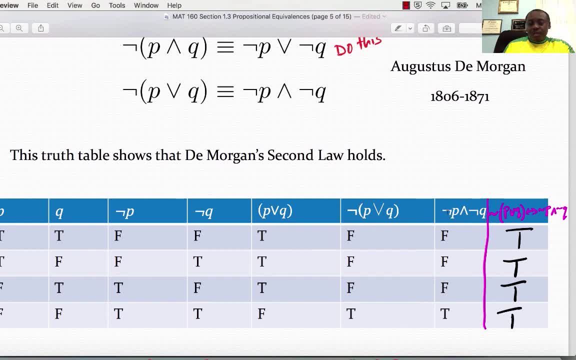 that that gives us f, f, f, t. and then we look at not p and not q. so here the two columns were interested in again, and it's only true if both truth values are t. so f, f is an f, f, t is an f, t, f. 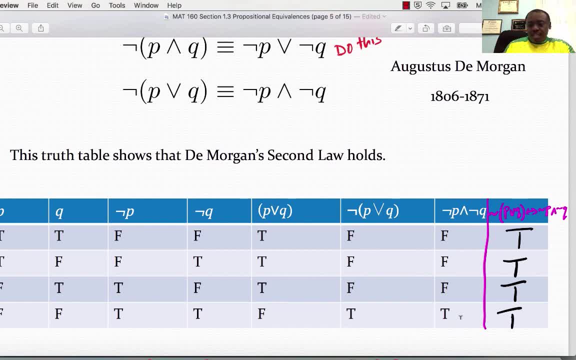 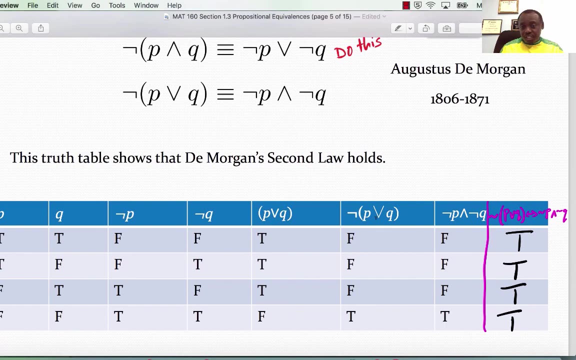 is an f, t, t is an f. both columns are the same. the truth values agree. so we can conclude that these two compound propositions are logically equivalent. or we can add a final column which is not p or q, if and only if not p and not q, and 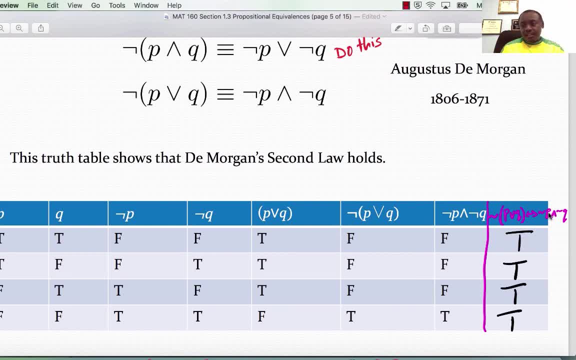 observe that we end up with a tautology again. this is true if, and only if, both truth values are t. so we have f if, and only if f is t. f if, and only if f is t. f if, and only if f is t. t if and only if t is. 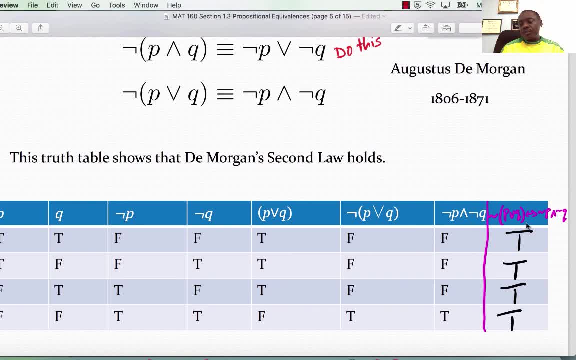 t, so we have a tautology and Therefore we can conclude that these two propositions are logically equivalent. So I think, as far as truth tables are concerned, we know how to verify that two compound propositions are logically equivalent. Is there any other way to verify logical equivalence without using truth tables? 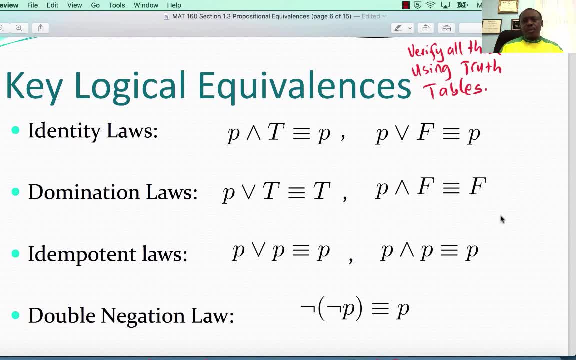 Before we get there, let's go ahead and give you some very important, useful logical equivalences. We call them key logical equivalences And, yes, you are welcome to use some of these when you're proving logical equivalences, because these are already done, have been proven. 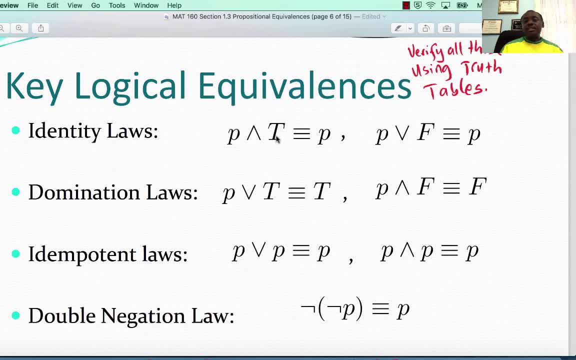 And the whole the identity laws, P and T. it doesn't matter what P is. P and T is always equivalent to P. P or F is equivalent. And we have the domination laws, We have the idempotent laws, We have double negation laws. 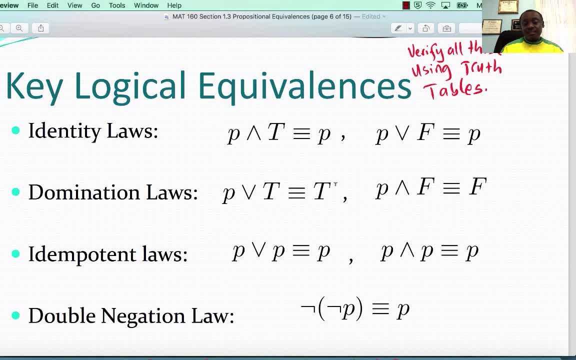 Not P, it's P And you can verify all of this. You can actually construct truth tables and verify each of these. I'm not going to ask you in a test to state the identity laws or the domination laws or the idempotent laws. 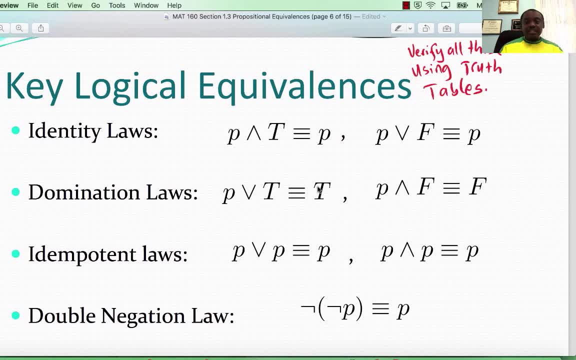 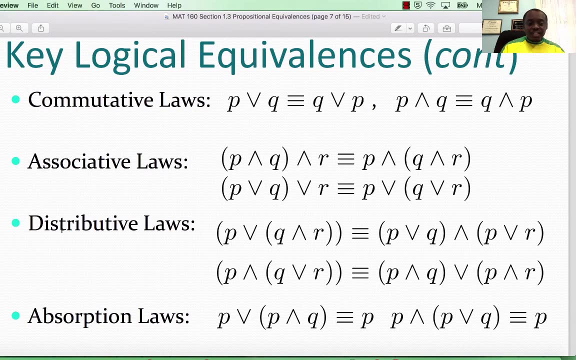 But I do expect you to know these laws and to be able to use them and apply them in solving problems. We will see an example as we move on. Some more logical equivalences: Commutative laws, Associative laws, Distributive laws. 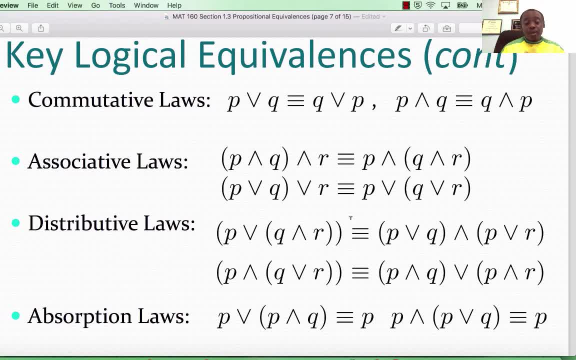 Absorption laws. Verify these. I'm going to ask you to do some of these in class, But I expect you to verify them yourself even before you get to class. For example, the distributive laws: You want to verify that P or Q and R is logically equivalent to P or Q. 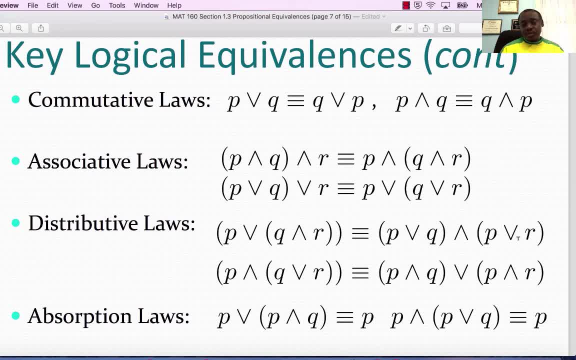 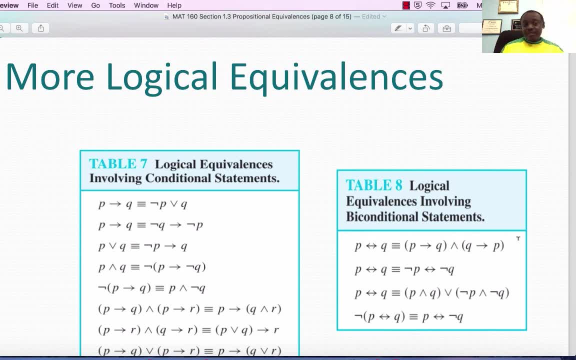 And P or R and so on and so forth And even more. These ones are actually very interesting and I need you to remember at least a couple of them. For example, you should be able to know that P implies Q is logically equivalent to not P or Q. 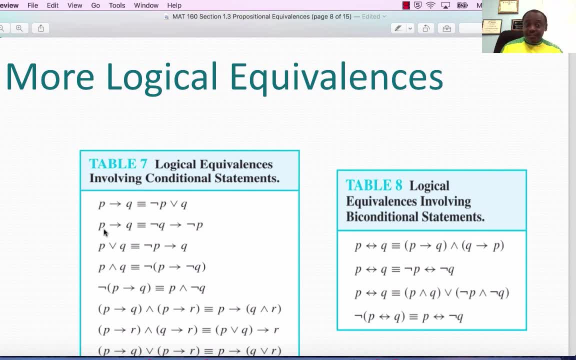 We already proved this using truth tables And, as a matter of fact, P implies Q is also logically equivalent to not. Q implies not P. Remember our contrapositive thing. So there are so many of them, You just need to go through these. 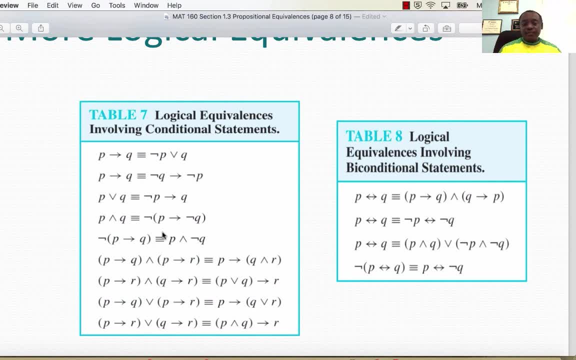 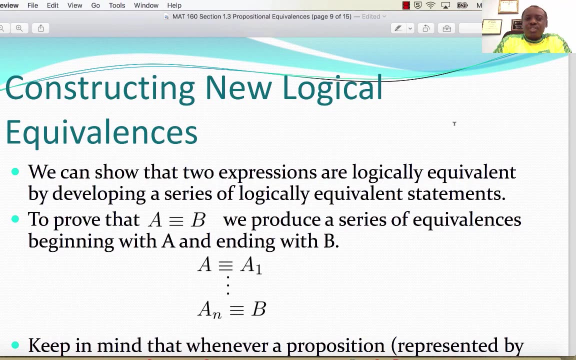 I might give you some of these tables in a test for you to use when you're proving logical equivalences, But I need you to know how to at least use these known key logical equivalences. Okay, let's look at constructing new logical equivalences. 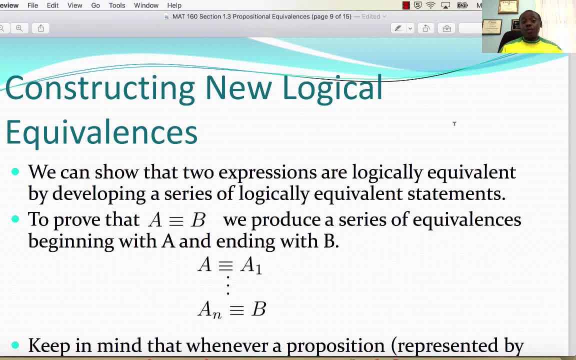 We can show that two expressions are logically equivalent by developing a series of logically equivalent statements. Remember, I did Say that you can verify the logical equivalence of two compound propositions by using a truth table, Or you could do that in a different way. 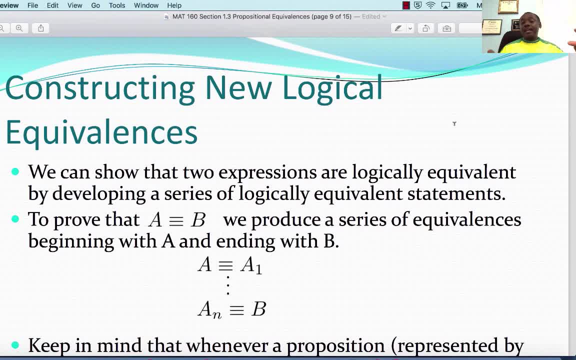 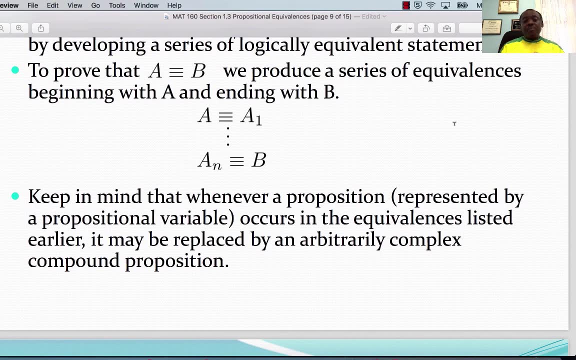 And this is the different way To prove that A is logically equivalent to B. we would produce a series of logical equivalences beginning with A and ending with B. That's going to be fun. Okay. now, as we proceed, I want you to keep in mind that whenever a proposition 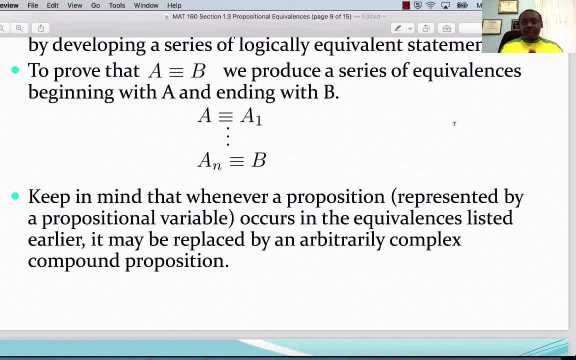 represented by a propositional variable. for example, P implies Q occurs in the equivalences that we've listed. above all those many key logical equivalences, each of those propositional variables can be replaced by an arbitrarily complex compound proposition. So when you see P implies Q, it could be a huge complex compound proposition. implies another complex compound proposition. 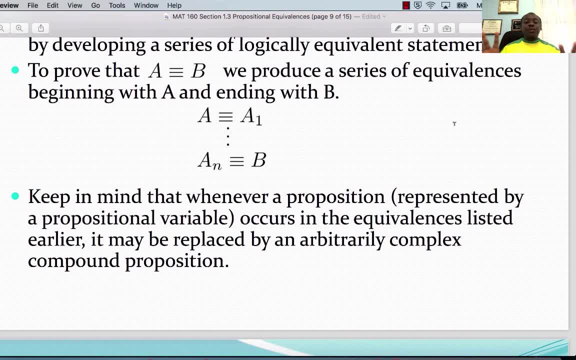 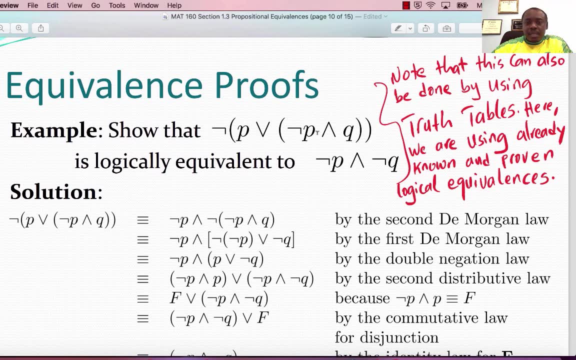 All you have to do is apply the key Logical equivalences and go from A to B without breaking your leg, without making an error. Let's try a few of those. Example one: Show that not P or parentheses, not P and Q is logically equivalent to not P and not Q. 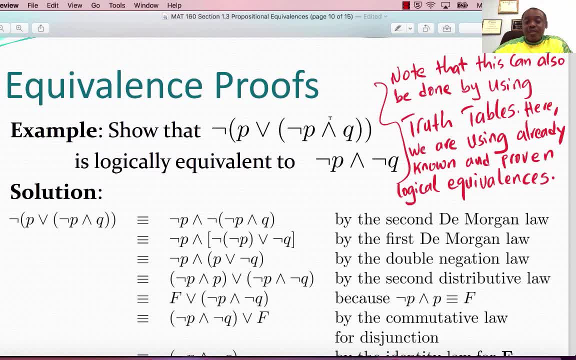 Again, you can use two tables to get this done, But here we expect you to prove that this compound proposition is logically equivalent to not P and not Q. Again, you can use two tables to get this done, But here we expect you to prove that this compound proposition is logically equivalent to not P and not Q. 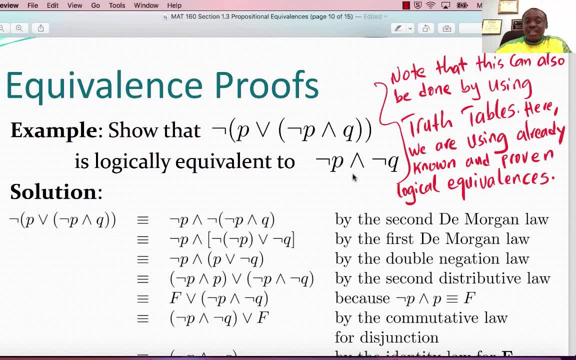 Again, you can use two tables to get this done. Again, you can use two tables to get this done, But it is logically equivalent to the other one without using two tables. Use a series of logical equivalences, So let's start. 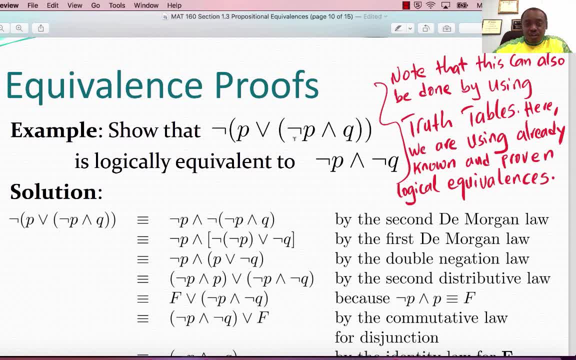 So we start with the left hand side, right here, It's a lot easier to break down a house than to build one. So we start off with this- that looks really huge, and break it down to not P and not Q. So we start off with this- that looks really huge, and break it down to not P and not Q. 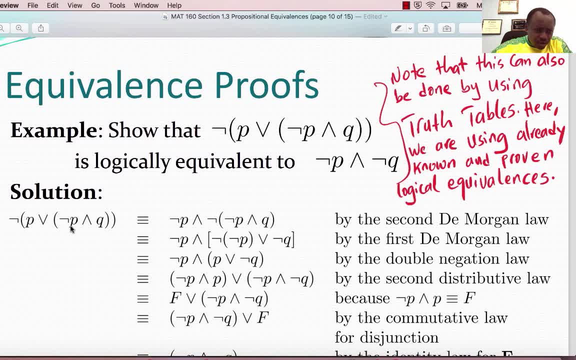 So we start right here, And what is it that we see? Oh wait a minute. De Morgan's Laws, sign p gets negated, the all becomes and, and all of these gets negated. and then i can take the negation for that in apply demogons again, and so on and so forth. so we apply demogon first, and that. 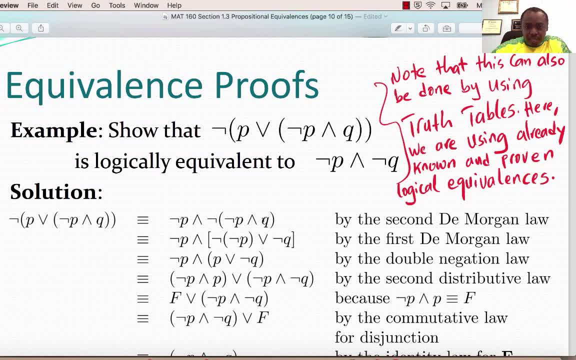 gives us not p and not into, not p and q. that's good. we leave the left component all by itself, the and still stays. i distribute my negation again using demogons: the first component gets negated, the and changes to all, and the second component also gets negated. so that gives us: 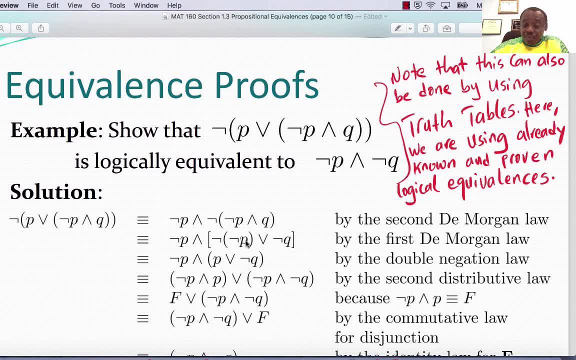 not, not p or not q. but wait a minute, not not p. is p one of the key logical equivalences. so that gives us not p and right here, p or not q. so what do we do from here? oh, wait a minute. the distributive laws. we can distribute these and it gives us not p and p, or not p and not q. wow, 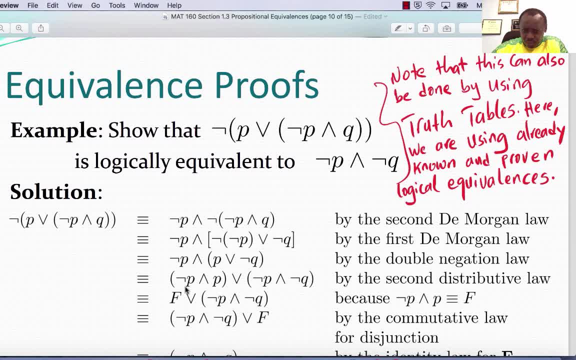 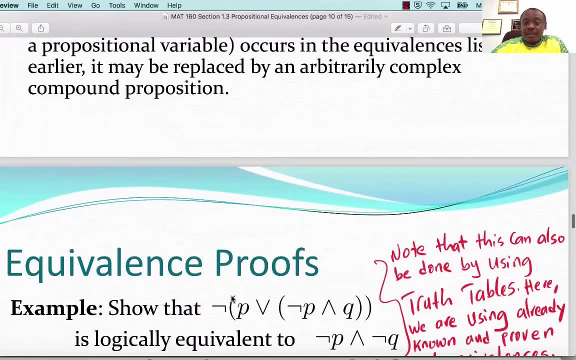 you? that's beautiful. wait a minute. uh, what else? what else? what else? oh, not p and p is always false. that's a contradiction. so that is f or not p and not q, but f or something gives us what. let's go back and look at it. f or a proposition is the proposition. it doesn't matter how complex the 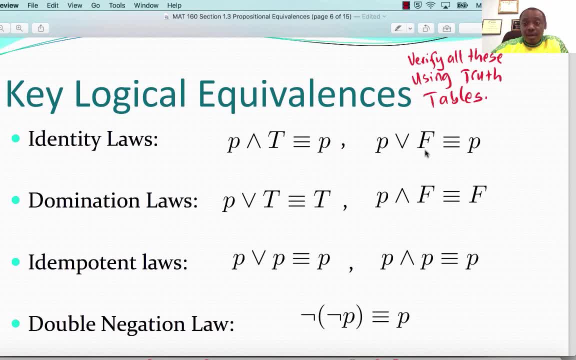 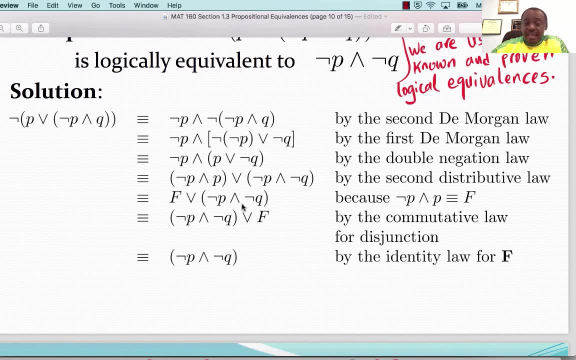 proposition. is that compound proposition or false is always the proposition. so let's go back to our problem. all of this or that, and you could see that if we really want to make it look exactly like the key logical equivalence we just looked at, we can use our 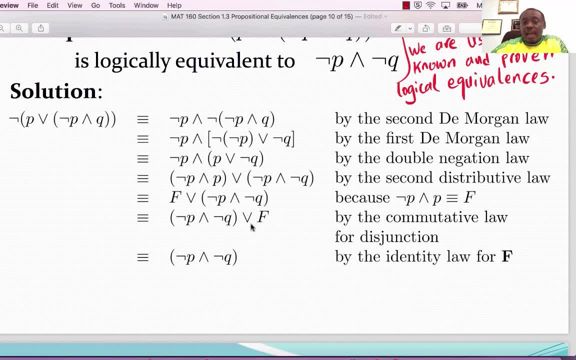 commutative law to flip this around, and then we apply that key logical equivalence and we end up with not p and not q, which is exactly what we are trying to prove, and we are done so if you are given a problem in this class and you are asked to verify that two. 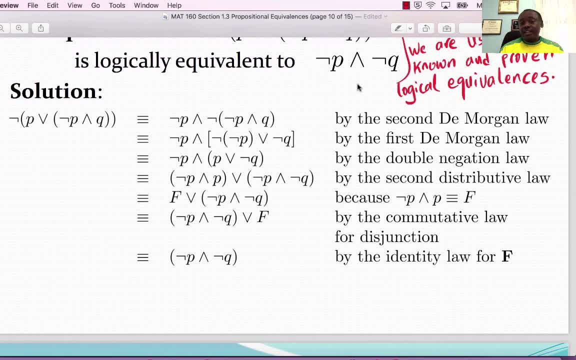 compound propositions are logically equivalent. you can do that either by using truth tables or you can do that using a series of logical equivalences. but of course, if i specify that, use truth tables, you have to use truth tables, and if i specify that, do not use truth tables. 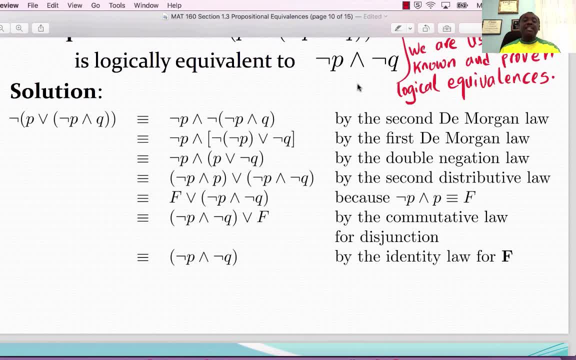 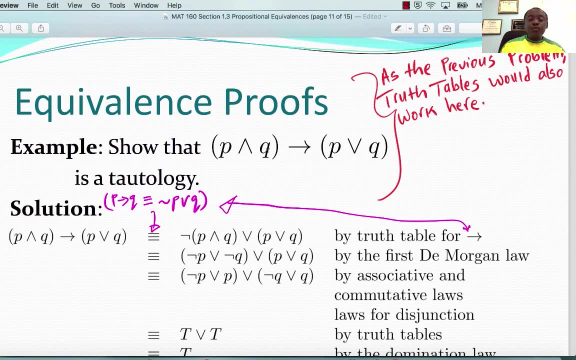 instead use a series of logical equivalences, then i expect you to do it exactly like this. i think we need one more example. example two: prove that p and q implies p or q is a tautology. again, you could use two tables, except you are asked. 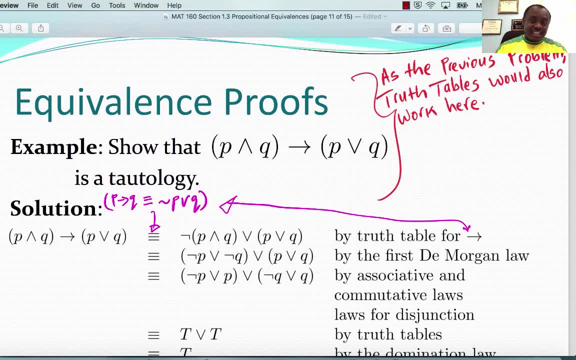 precisely not to do that, or you could use a series of logical equivalences. in this case, we are using a series of logical equivalences. so what are you actually asked to prove? to prove that this is a tautology? you are basically proving that the very last column would give you all 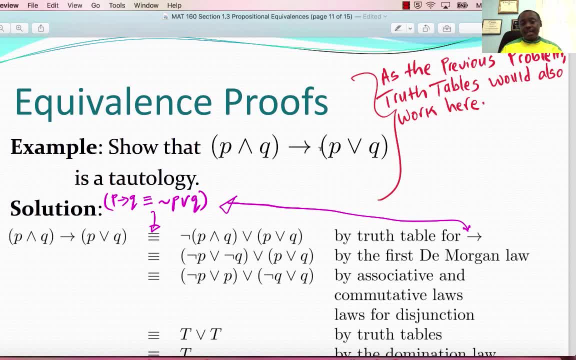 true, that is, if you use two tables. but let's go ahead and look at a series of logical equivalences. solution p and q implies p or q. so we get stuck right here. how do we proceed? then? we remember that p implies q is logically equivalent to not p or q. in this case, that is your p, all of this, your p and all that's. 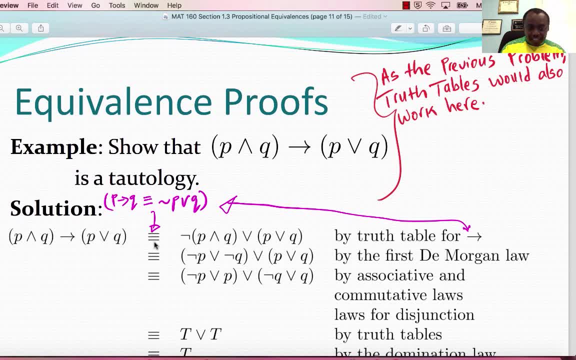 a q. so all of this implies all of that is logically equivalent to, not the first component, the second component. now the morgan comes in, the morgan goes in. we have not p or not q, or p or q. that's very good. and from here all we have is all, all, all. we can move things around by associativity. 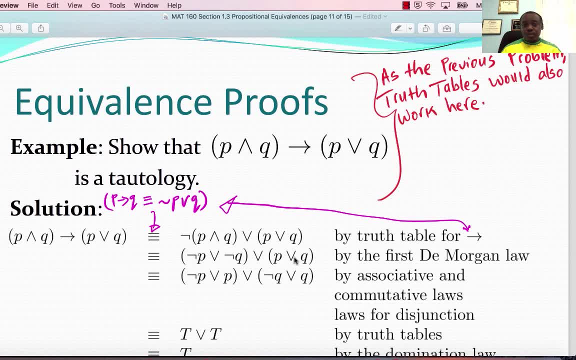 we can move things around by commutativity. we can do just whatever we want to do because it's all all. so we move this p around. we end up with not p or p, or not q or q, but not p or p is true, not q or q is true. both are tautologies. so we end up with t or t and t or t is always true. 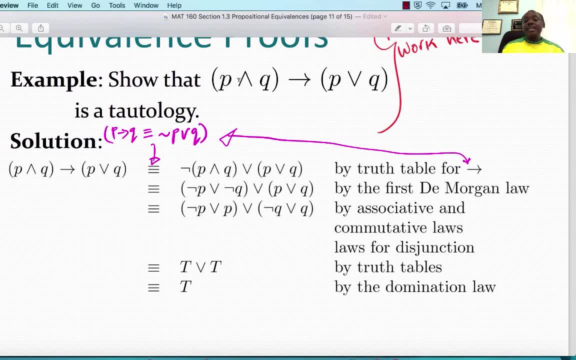 what have we done? we've successfully shown that p and q implies p or q is a tautology. it's always true. this whole concept introduces you very slowly to the concept of proofs. we would use this same idea to prove a couple of things in set theory, and if you 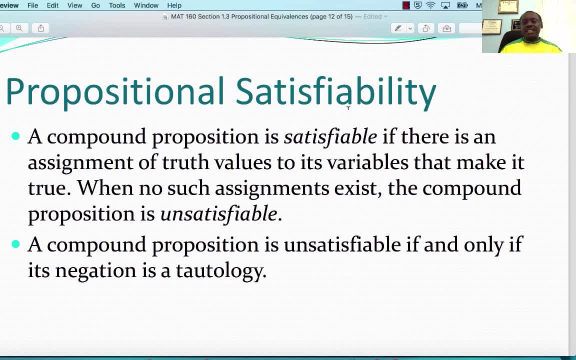 play the find the rule ofMi the wrong understanding. the problem is, we can tested bene this approach and if that so, you have this prediction of a set theory and we do. still an example of proofs. it just may have to say this the other way around. let's just say, in set theory, if you get an equation when one of thesešum can popped, 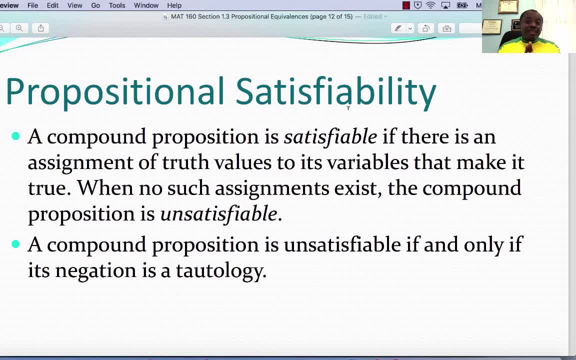 one of the interesting techniques that we found in set theory is the verification of what is a security function and then proving to others that it's a security function. then it's absolutely a security function. y's farkman doesn't have to kick you off the compound proposition. true, when no such assignment exists, the compound proposition is. 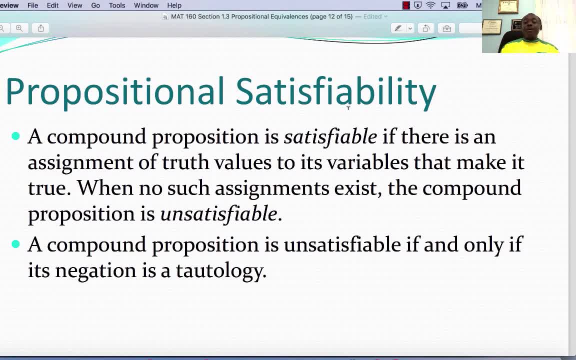 unsatisfiable. so a compound proposition is unsatisfiable if, and only if, its negation is a tautology interesting. so if i give you a compound proposition and ask you to prove that it is unsatisfiable, well, you could check all possible combinations of truth values and show. 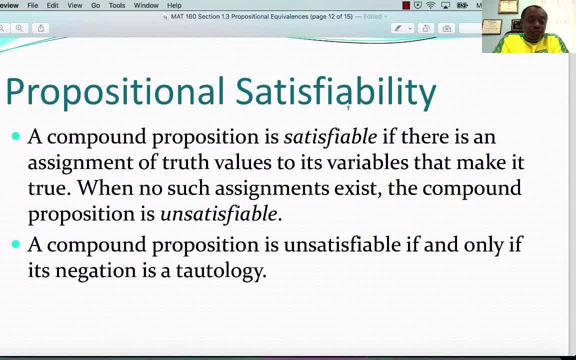 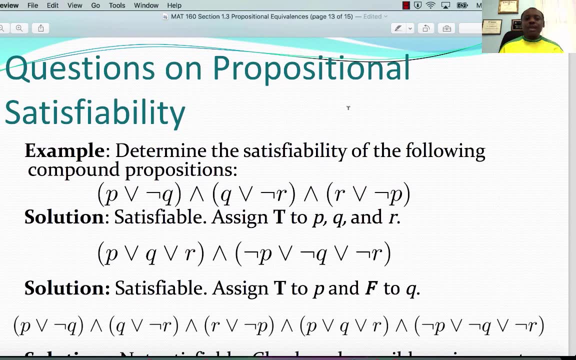 that there is no possible assignment of truth values to its variables. that will make it true. or you could just come up with a truth table and show that the negation of that statement is a tautology. that's beautiful. let's look at a few examples. example one: determine the satisfiability. 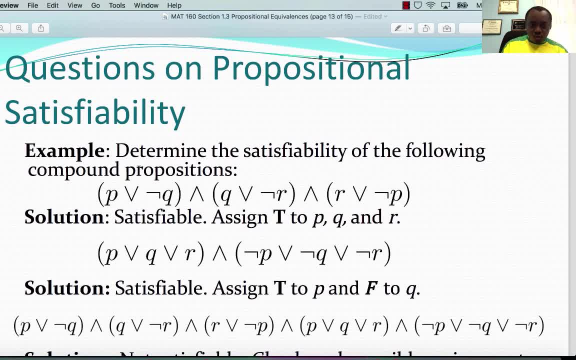 of the following compound propositions. the first one, right here: is it satisfiable or not? by observation, if we assign t to all three- p, q, r- then we end up with the compound proposition being true. so it is satisfiable. the second one, again: if we assign t to p and f to q, then this compound 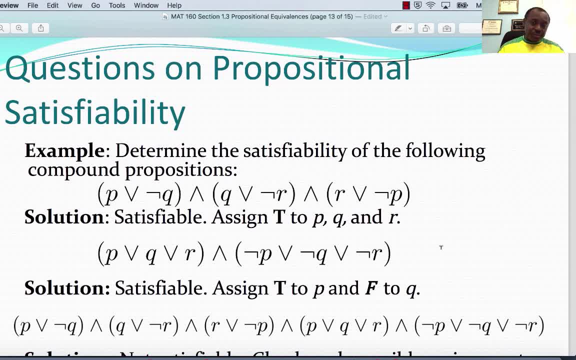 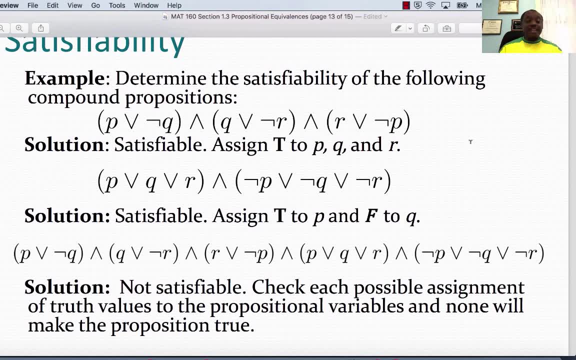 proposition ends up being true, so it is satisfiable. what about the last one? well, it is not satisfiable. and it is pretty tough to verify that, because you have to come up with all possible combination of truth values and show that no assignment of truth values to the propositional variables would lead to the proposition being true, or we construct a truth. 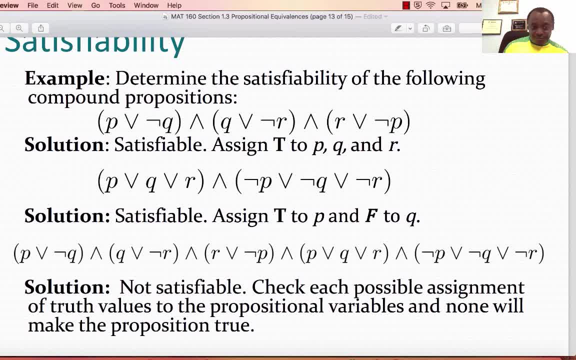 table and show that the negation of this entire compound proposition gives us a tautology that should probably give you an idea. if you are verifying the satisfiability of certain compound propositions- and it's a little bit difficult to come up with a conclusion- you may just want to do a. 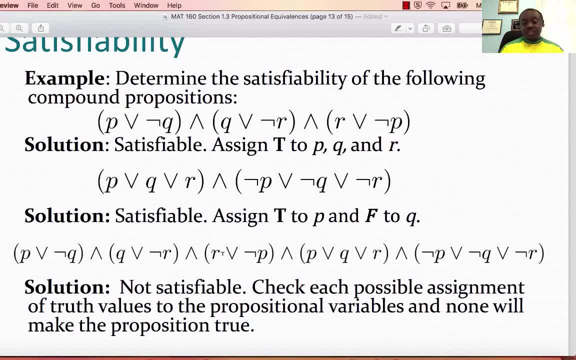 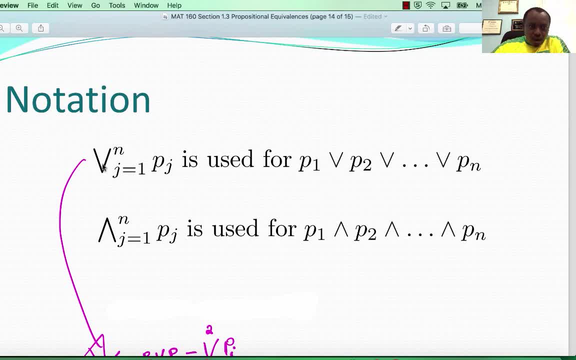 truth table and check the negation of the compound proposition. if it's a tautology, then we're done. now let me end with some notation. observe that this is just or j from 1 to npj. what this simply means is p1 or p2 or or pn. remember: j goes from one to n. j is just a dummy variable. same thing for: